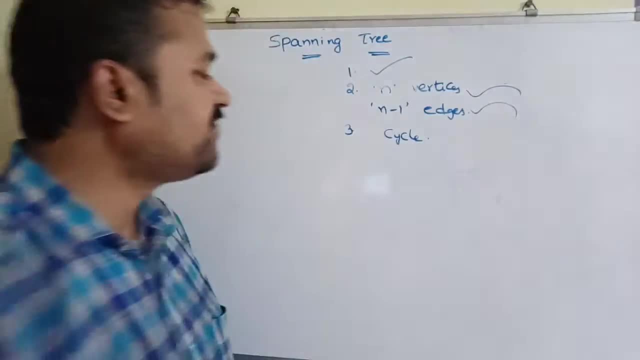 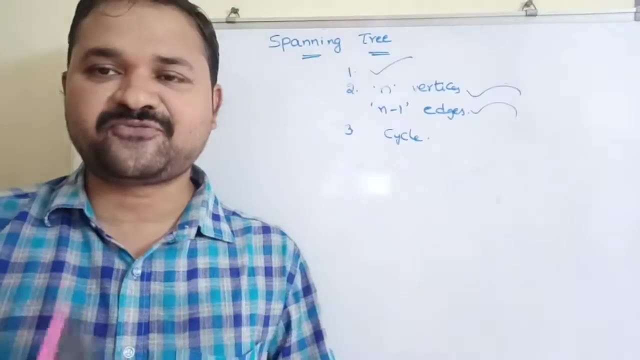 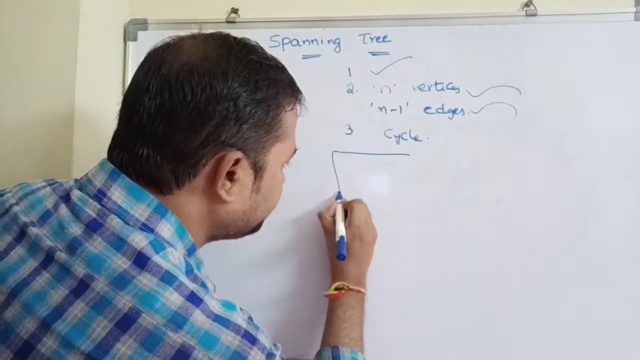 should contain n minus 1 edges. Third property: spanning tree should not contain any psyche. Now let us take a graph And let us try to construct various spanning trees from the corresponding graph. So let me have a graph like this: Let ABCD is the graph, So this: 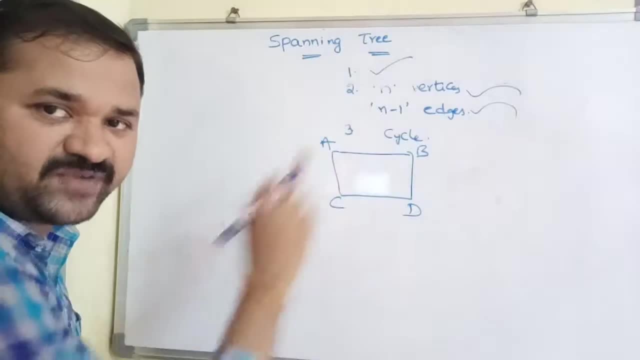 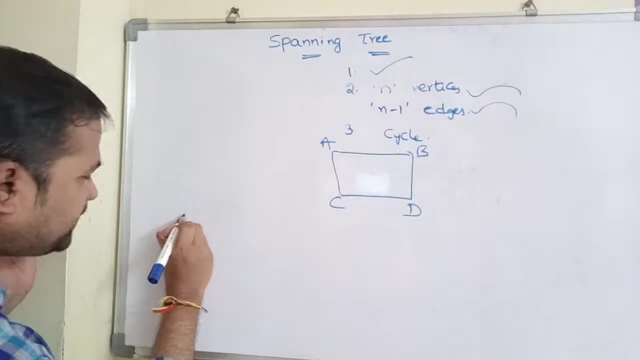 is our graph. So this graph contains totally 4 vertices. Now let us construct the possible spanning trees. So this is one of the three properties, So let us construct one of the which are derived from this graph. The first spanning tree is like this: 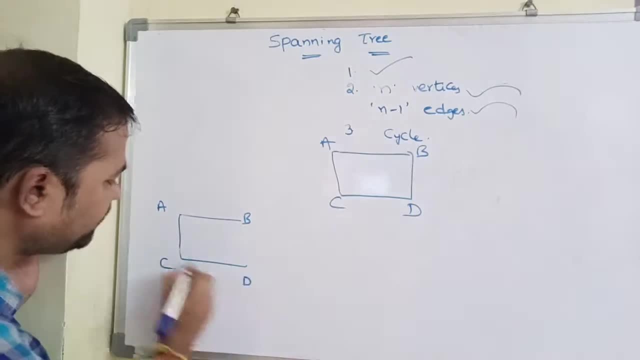 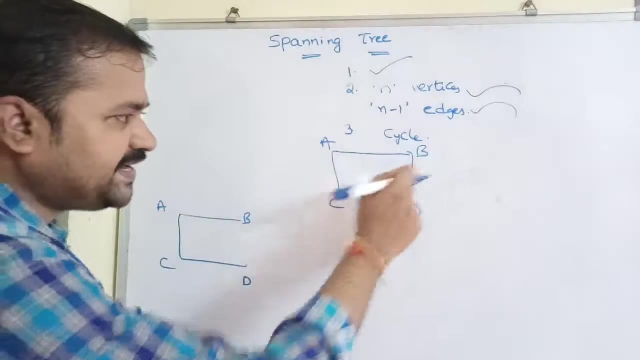 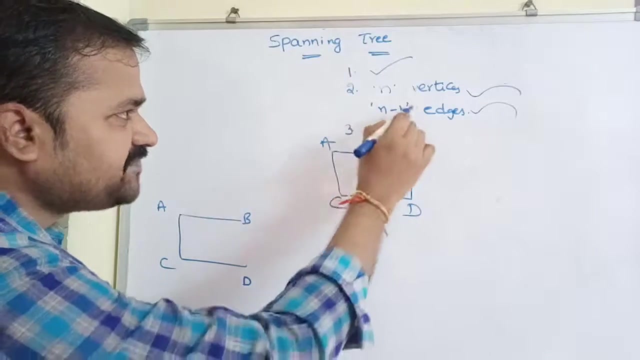 So a, b, c, d, So totally we have to satisfy three properties. What is the first property? It should contain all the vertices of the graph. Here the graph contains four vertices, So our spanning tree also contains four vertices. Second property: if the graph contains n vertices, 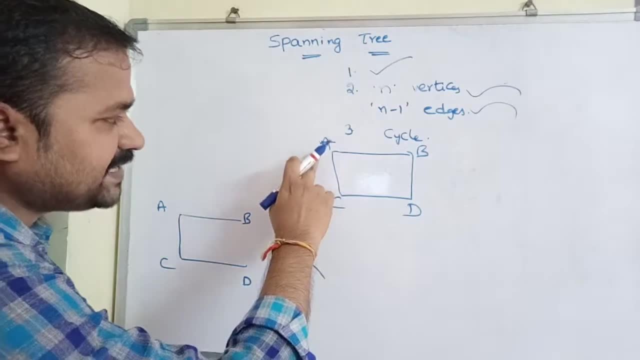 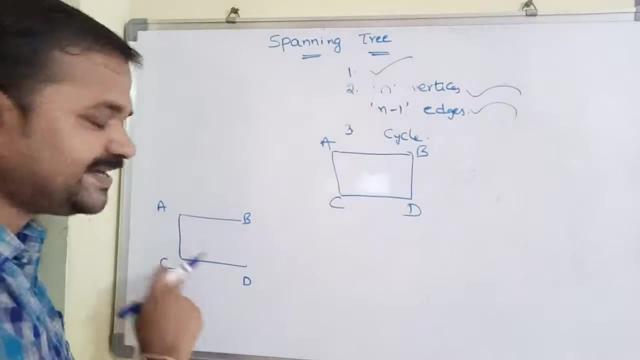 then the spanning tree should contain n minus 1 edges. Here the graph contains four vertices, So spanning tree should contain four minus 1.. That is nothing but three edges. So first edge, second edge, and third edge, Third property. it should not contain any cycle. Here we do not. 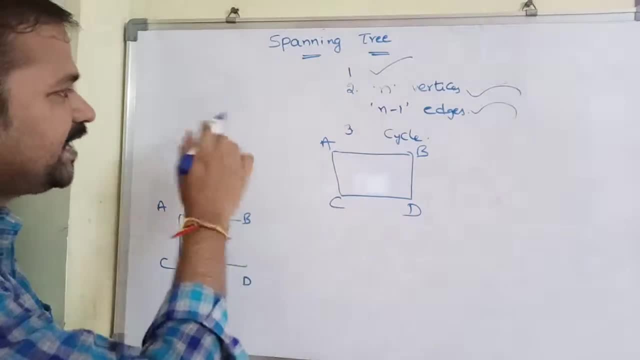 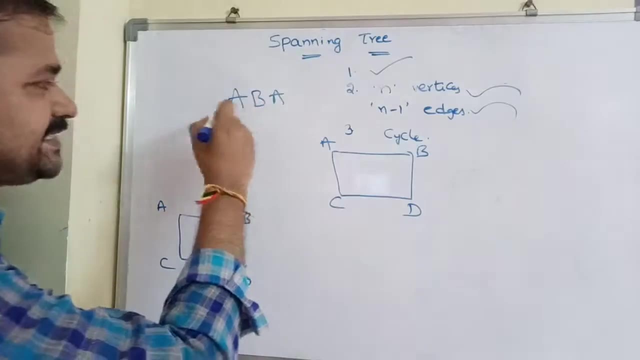 have any cycle. So what is a cycle? It is a path in which the starting vertex as well as the destination vertex are the same. So a, b, a, So this is a cycle. So this is a cycle Why? Because 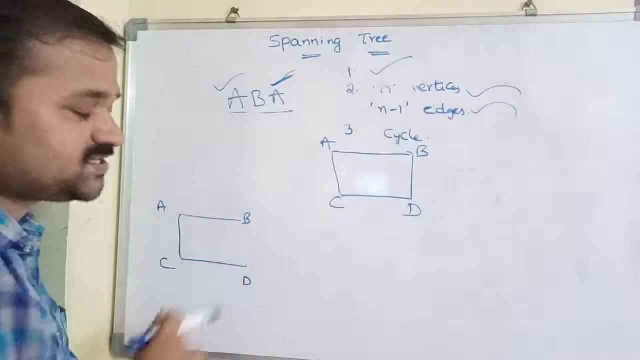 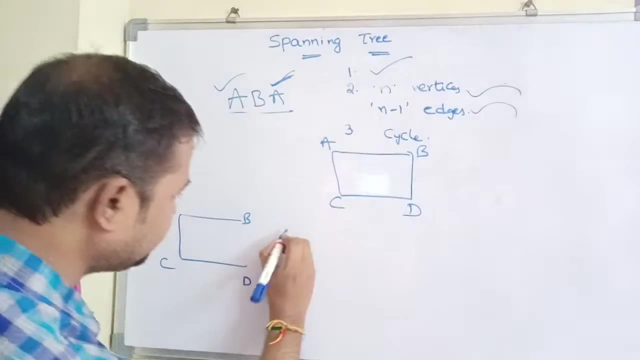 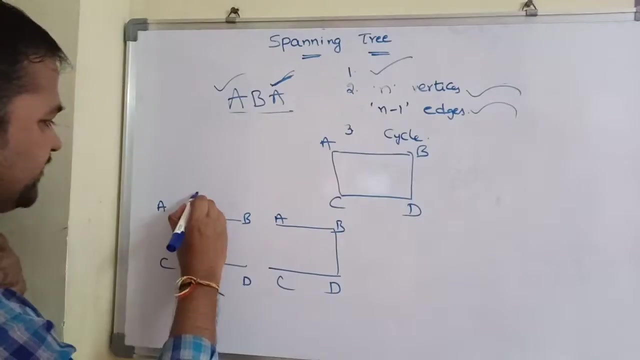 in this path, the starting vertex as well as the ending vertex are the same. So likewise, this spanning tree does not contain any cycle. So likewise, we can construct three more spanning trees, So we can write the next one like this: So a, b, c, d. So this is the first spanning. 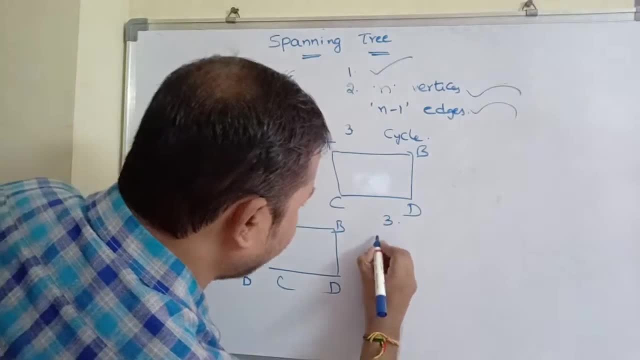 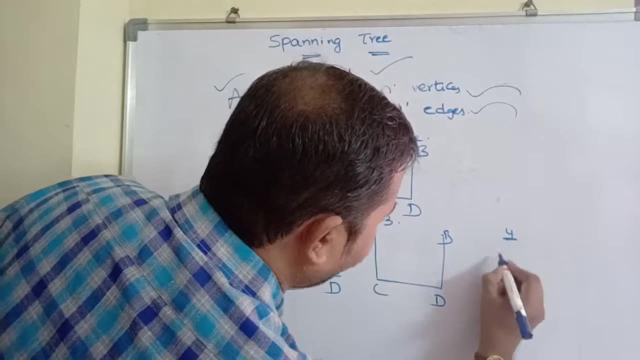 tree, second spanning tree. Now let us write the next spanning tree: So a, b, c, d. So this is the third one Next to fourth spanning tree. we can construct like this: So a, b, c. 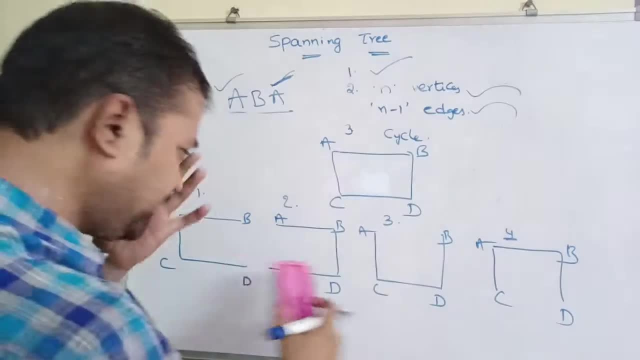 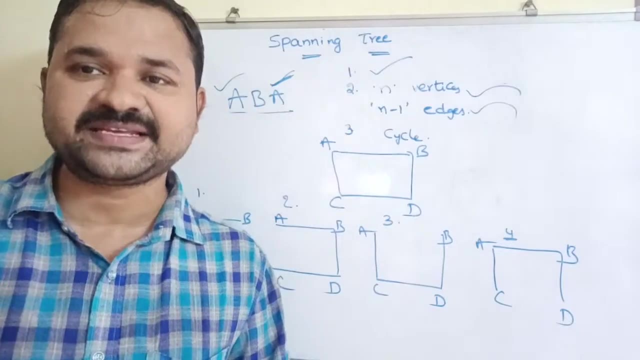 d. So from this graph, totally, we can derive the following: So a, b, c, d. So this is the same. We can construct four spanning trees. So this is about the definition and the properties of a spanning tree. Now let us see about minimum cost spanning tree. Now. 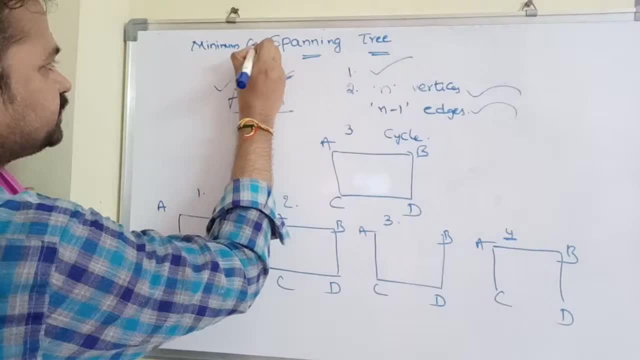 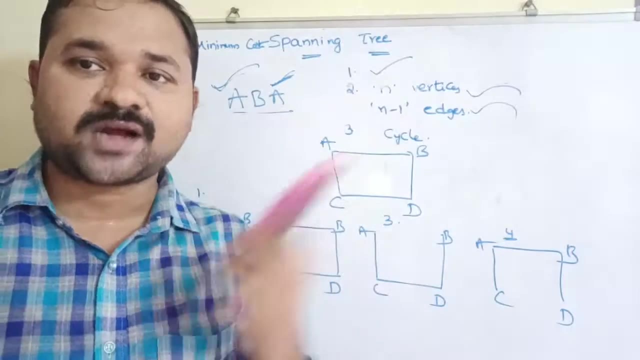 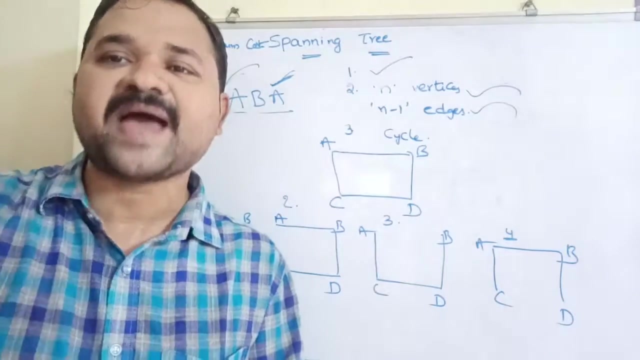 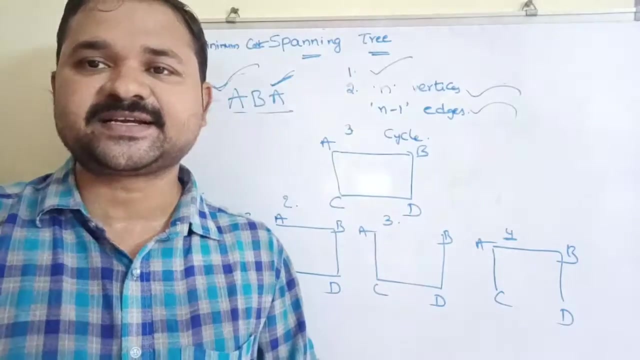 let us see about minimum cost spanning tree, A spanning tree in which the cost is minimum. So here the cost can also be called as weight. So if a spanning tree weight is minimum, then the remaining spanning tree, Then it is said to be minimum cost spanning tree or minimum spanning tree. So we can say that. 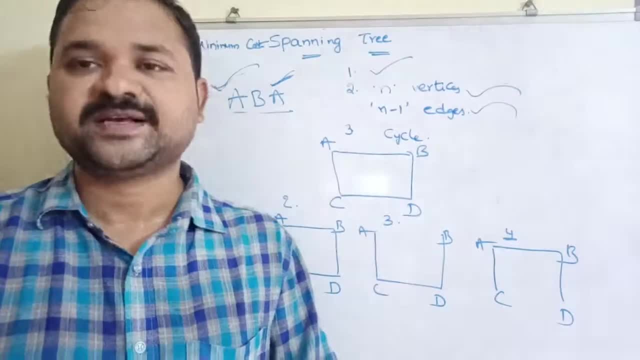 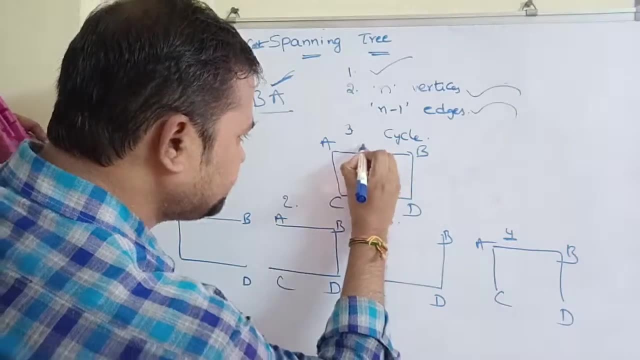 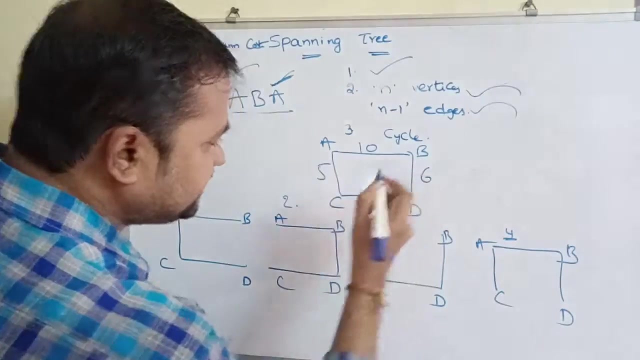 the cost of minimum spanning tree is minimum smaller compared with the remaining spanning tree's cost. Let us take this one. Let us assume that here the cost of this FG is 10.. The cost of this FG is- let us assume that it is 5.. It is some 6.. Let us assume that it is 3 here. So 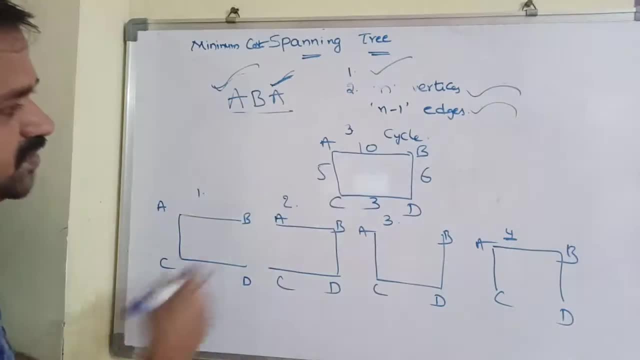 totally how many spanning trees We can construct here From this graph. totally we can construct 4 spanning trees. So this is nothing but cost 5,, 10,, 5,, 3.. Next, this edge cost 10.. We do not have any edge here. 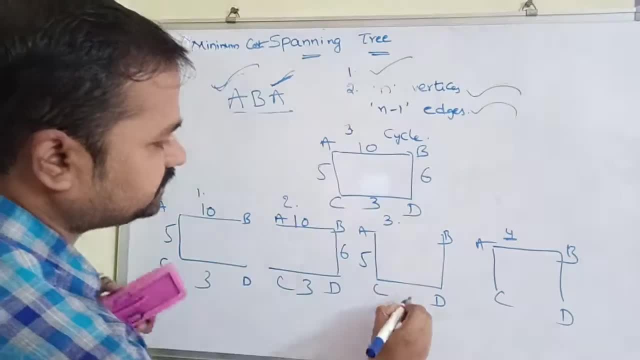 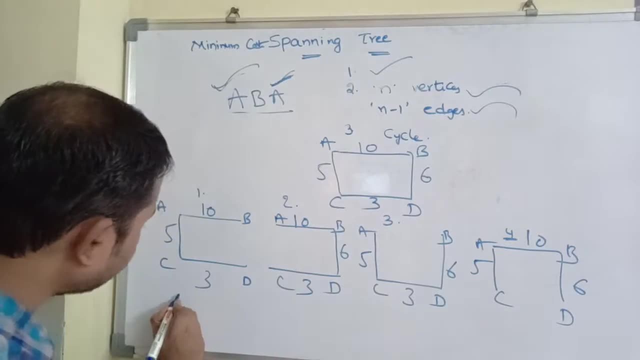 So 6, 3.. Next, this edge cost 5,, 3,, 6.. Next this one, 10.. So 5, 6.. So what is the cost of this spanning tree? So 10 plus 5,, 15.. 15 plus 3, 18.. 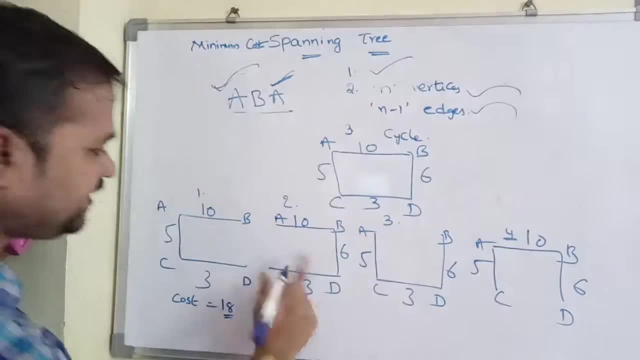 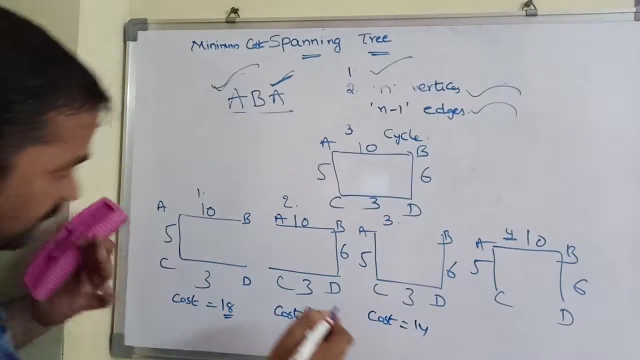 Cost of this spanning tree: So 10 plus 6,, 16.. 16 plus 3, 19.. Cost of this spanning tree: So 5 plus 3,, 8. 8 plus 6,, 14.. 14. Cost of this spanning tree: So 10 plus 5,, 15. 15 plus. 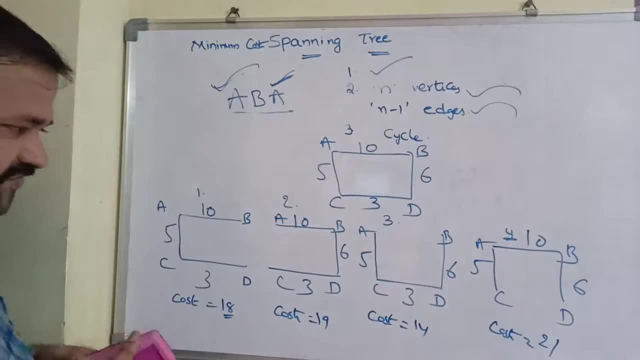 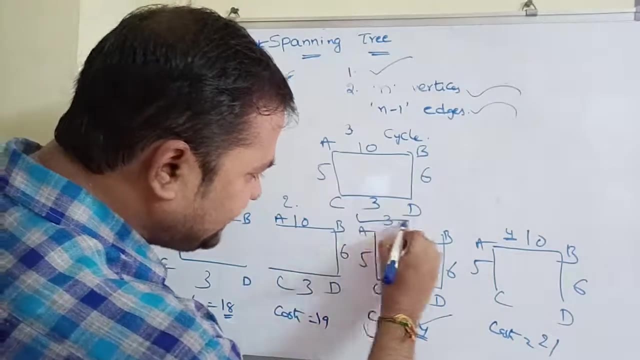 6,, 21.. So, out of all these costs, so which is the minimum cost? 14.. So this is the minimum cost. So we can say that this spanning tree, this spanning tree, is the minimum cost. spanning tree. 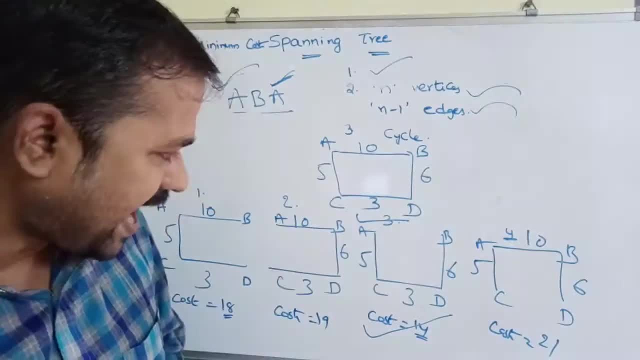 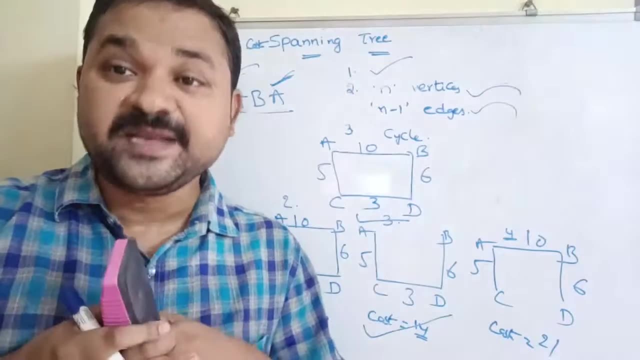 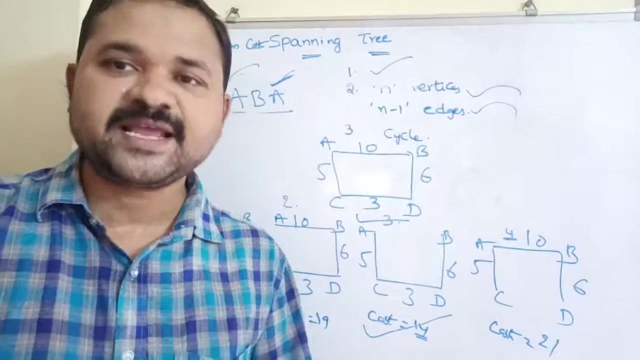 The remaining three trees. Why? Because this spanning tree has minimum cost than the remaining spanning trees. So this is about what is spanning tree and what is minimum cost spanning trees. In order to construct minimum cost spanning tree, we have two algorithms: Prim's: 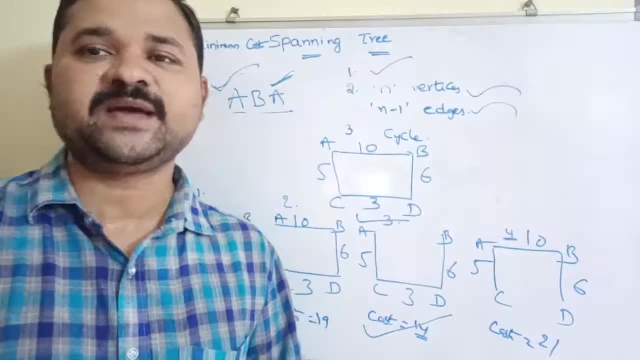 algorithm and Kruskal's algorithm. In the next videos we will see about those two algorithms.